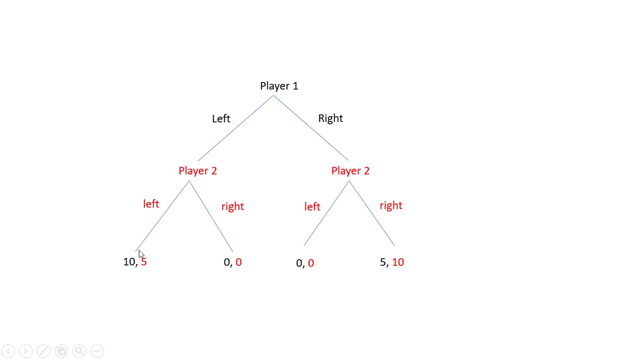 If player 2 plays left, player 1 gets a payoff of 10, and player 2 gets a payoff of 5, where bigger numbers are better here. If player 2 were to play right, player 2 would get 0, and player 1 would get 0. 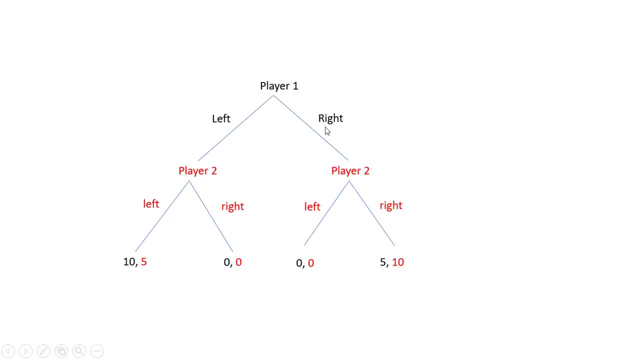 This game could also end up here, where player 1 would play right and ends up over here at this right node, far right node, for player 2.. And at this particular node, player 2 could play left. player 2 would get a payoff of 0, player 1 would get a payoff of 0. 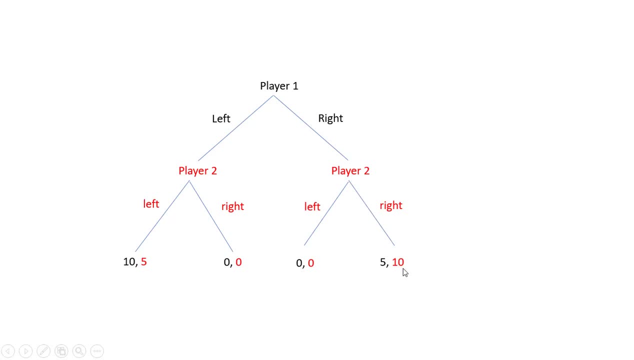 On the other hand, if player 2 played right, player 2 would get a payoff of 10, leaving player 1 with a payoff of 5.. So what we want to do is we want to solve for the equilibrium of this game, or the sub-game- perfect equilibrium. 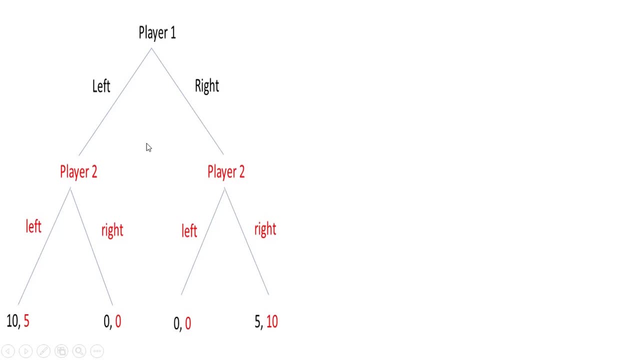 So here again is our game, our sequential game: Player 1 goes left, Player 2 goes first, And then player 2 makes his or her choice. So we're going to solve for this sub-game perfect equilibrium by something called backwards induction. 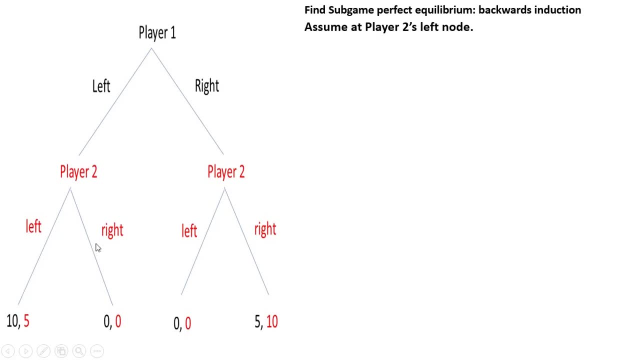 And we're going to start basically not at the beginning of the game, but basically sort of at the end of the game. So we're going to assume we're at player 2's left node. What is that? That means we're going to be over here. 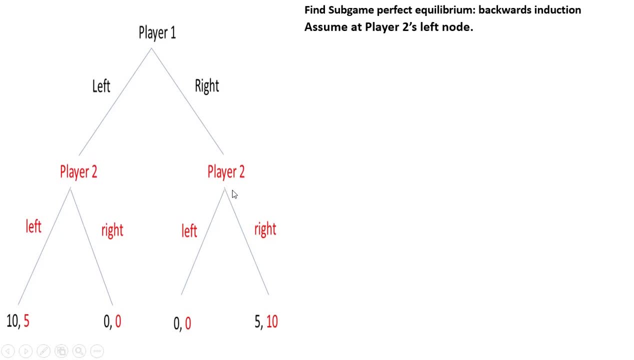 Here's node 1 for player 2 and the other node for player 2.. We're going to be at the left node. If this game were to end up here, what would player 2 do? Well, player 2 wants to get the highest payoff. 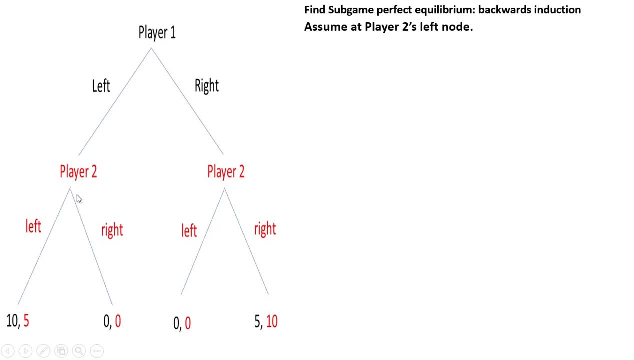 If player 2 goes right, player 2 gets 0.. If player 2 goes left, player 2 gets 5.. So player 2 only cares about his payoff. So if the game were to end here, player 2 would choose left. 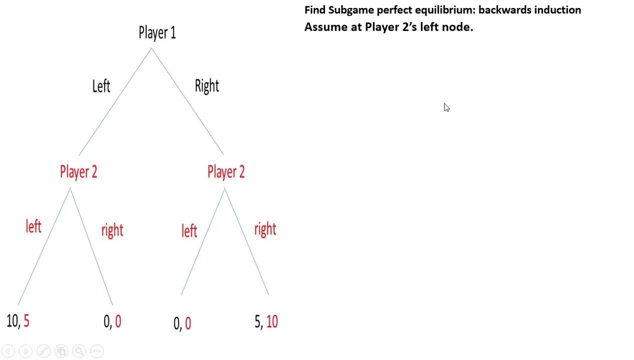 Player 2 would get a payoff of 5. And player 1 a payoff of 10.. So, as we just stated here, player 2 will choose left. A payoff of 5 is better than a payoff of 10.. Better than a payoff of 0 for player 2.. 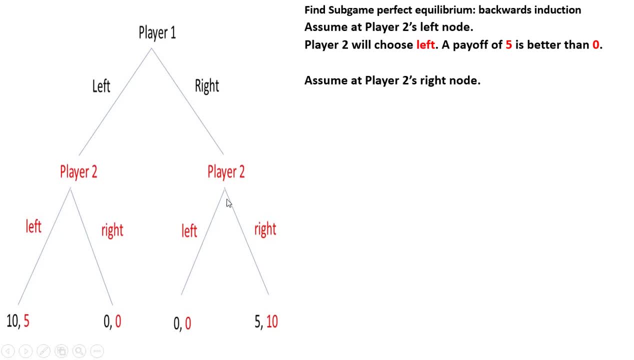 Now let's assume that we're at player 2's right node over here. What would player 2 choose to do in this case? Again, player 2 wants to get the highest payoff. If player 2 chooses right, player 2 gets a payoff of 10.. 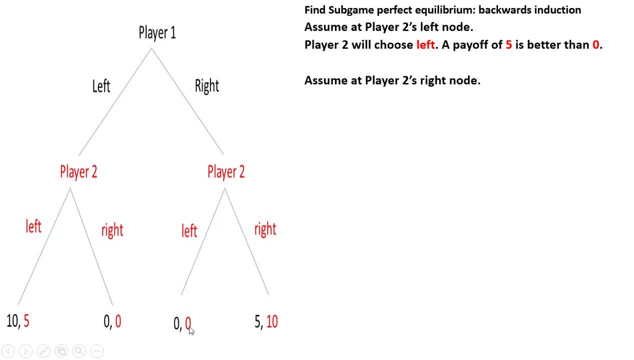 This number in red. If player 2 went left, player 2 would only get a payoff of 0. So 10 is bigger than 0.. Player 2 prefers bigger numbers. So if the game were to end up at this right node here, player 2 would play right. 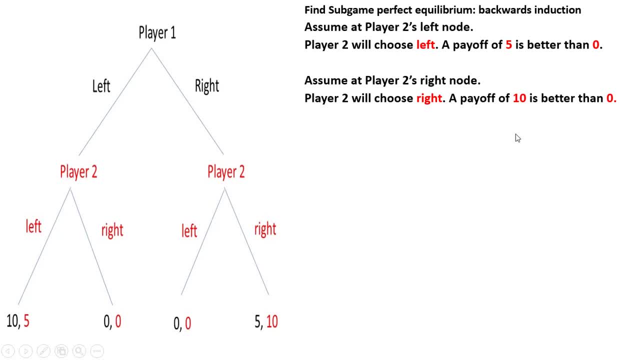 So player 2 will choose right. A payoff of 10 is better than 0. Player 1 knows how player 2 will respond. If player 1 plays left, player 2 plays left And that would give a payoff of player 1 of 10.. 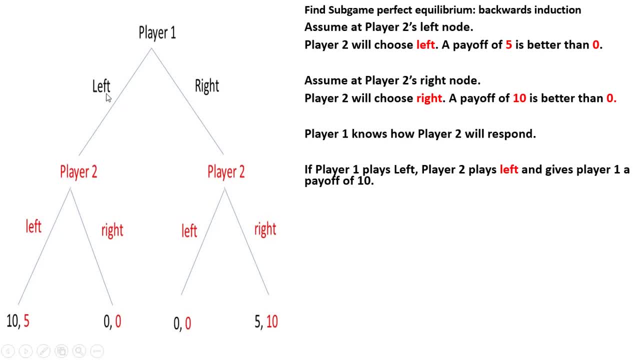 So player 1 knows that if player 1 plays left, player 2 will play left And in that case player 1 would get a payoff of 10.. On the other hand hand, player 1 knows that if player 1 played right- if he played right- player 2 would. 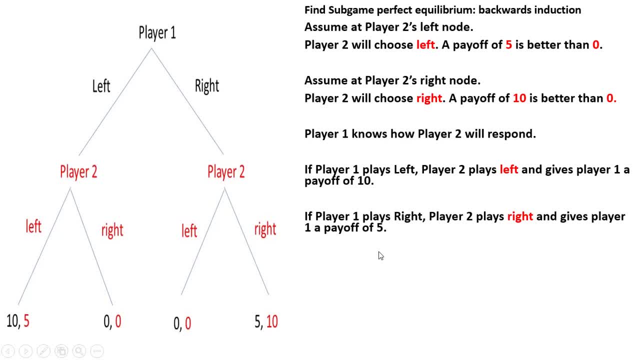 also play right, and in this case player 1 would get a payoff of only 5.. So what does player 1 want? Player 1 wants the highest payoff and that is going to be by playing left. So player 1 prefers 10 to 5, so player 1 will play left. Game ends up in this: left. 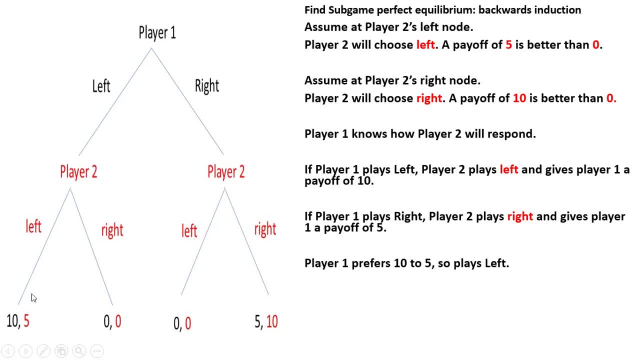 node here. Player 2 would then choose left, and that is going to be our sub-game. perfect equilibrium: 10 and 5.. 10 for player 1, 5 for player 2.. This is also a Nash equilibrium. Neither player has an incentive to change its strategy, given the other player's strategy. 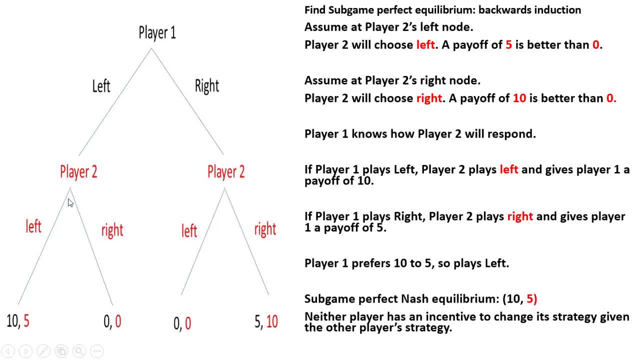 So, given that player 1 played left, player 2 wouldn't want to change their strategy to right. Okay, and likewise for player 1.. Player 1 wouldn't want to change their strategy from left, given what player 2 is playing. 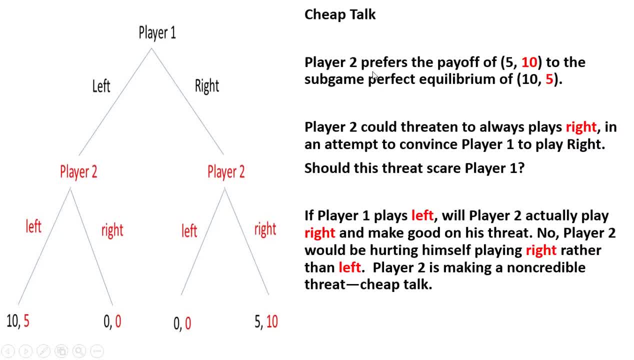 All right. one other thing I want to talk here briefly about is cheap talk. Player 2 prefers this payoff over here of getting 10 instead of 5, so player 2 may try to convince player 1 to change his strategy. So player 2 could threaten to always play right in an attempt to convince player 1 to. 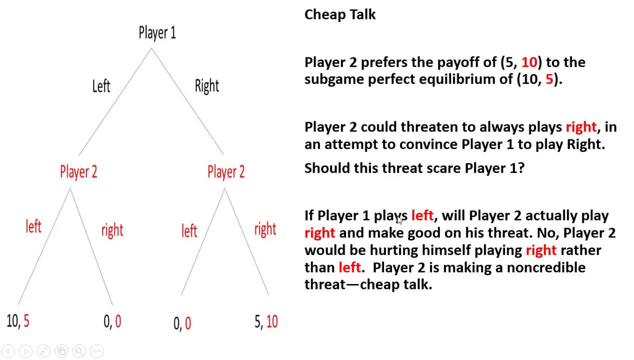 play right, should this threat scare player 1.. So here's sort of the idea. Player 2 says I'm always going to play right. so player 1 goes okay, if I play left and player 2 plays right, because player 2 is always going to play right, I'm going to get 0.. Well, that's. 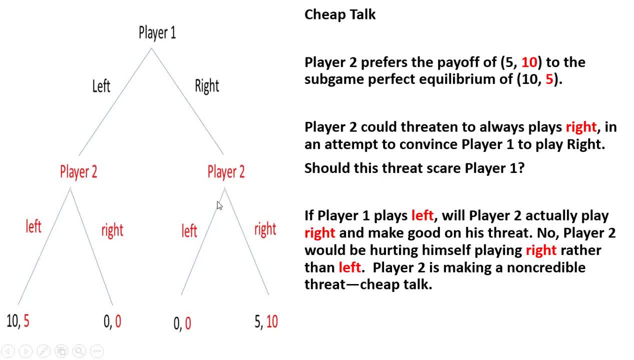 no good, If player 1 plays right, player 2 is always going to play right. then I'd get a payoff of 5 as player 1.. So player 2 says, I'm always going to play right, so player 1.. And since 5 is better than 0,, player 1 then says, well, okay, I'm going to play. 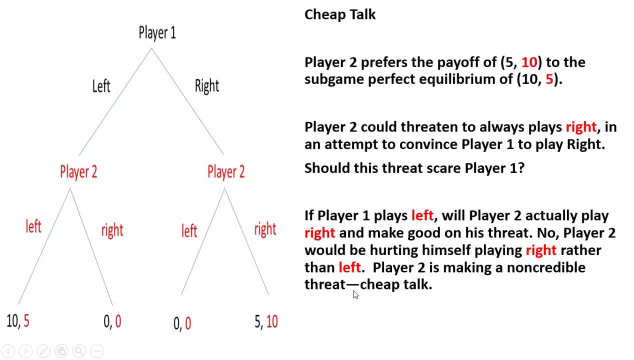 right, then I don't want to get 0.. However, we're going to argue this is a cheap threat. If player 1 were to play left, will player 2 actually play right? So if player 1 played left, if player 2 plays right, player 2 is they're harming themselves. They could have 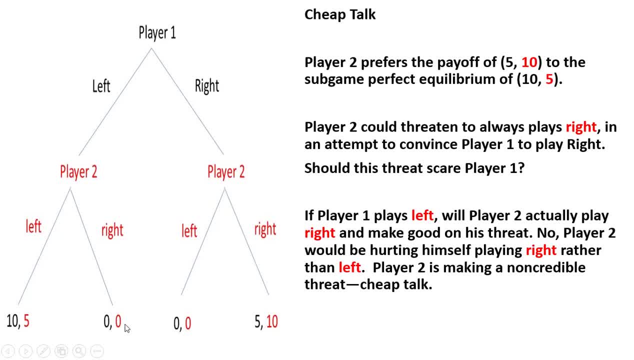 played left and got 5, but instead they played right and got 0. So this is really cheap talk. This is a non-credible threat. Player 2 will not play right if player 1 plays left, because player 2 will be hurting itself. So player 1 can ignore that threat. 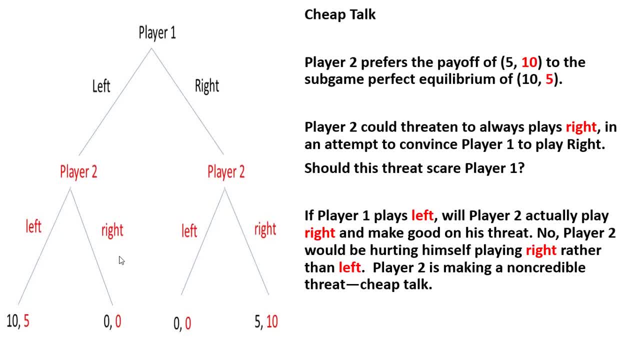 It's a non-credible threat. Alright, that's it. I hope you found this video helpful. 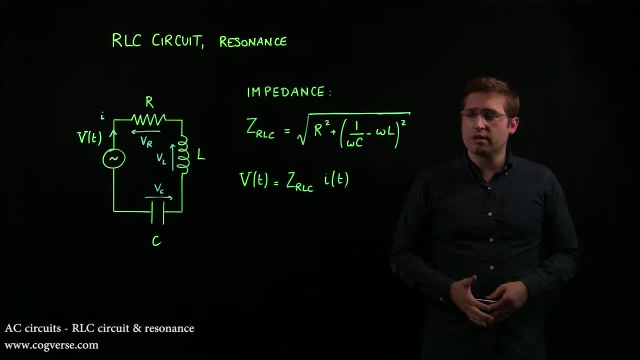 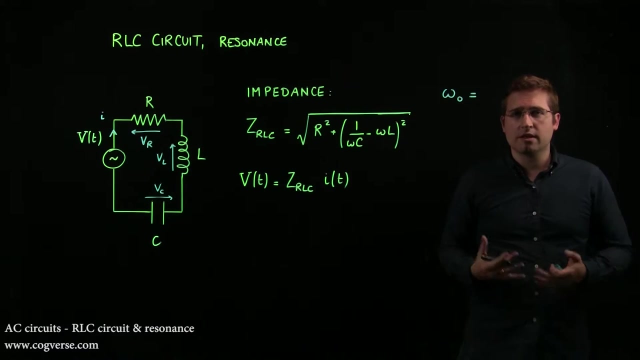 Now that we've defined the impedance of an RLC circuit and we've stated that it is a function of the angular frequency omega, let's see what happens when omega takes on a very specific value. If you remember the LC circuit, we said that it has a characteristic angular frequency omega naught equal to 1 over root LC.